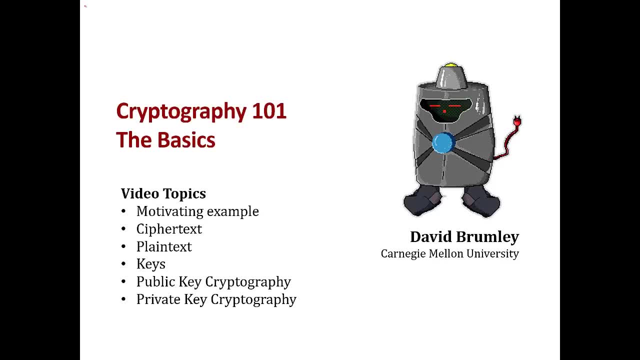 scene where we want to use cryptography. I'm going to use this to explain a basic vocabulary like what a ciphertext is, what plaintext is, what are cryptographic keys, And then I'm going to describe a little bit of what public key cryptography is and what private key cryptography. 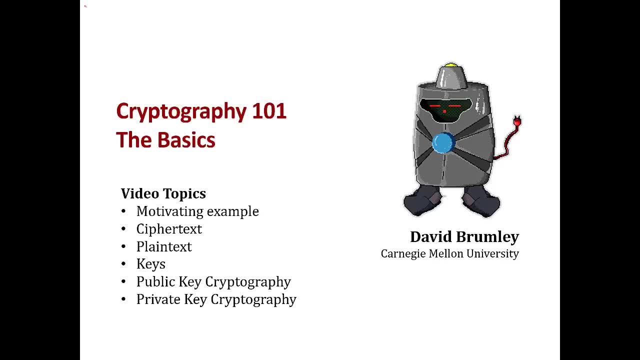 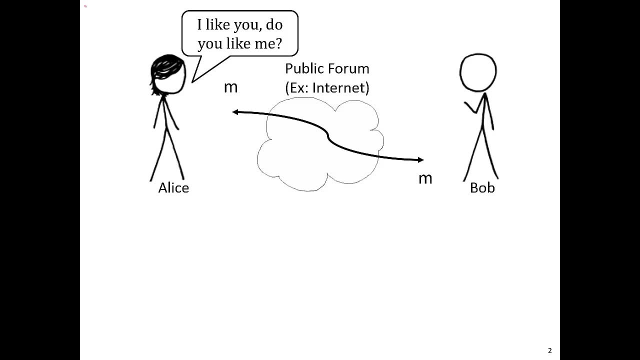 is. I want you to really just have an understanding of these terms. So we start out with the following motivating example: In this example there's two people, Alice and Bob, that want to talk And they want to pass notes back and forth, and these notes are private. For example, Alice, maybe, is wanting 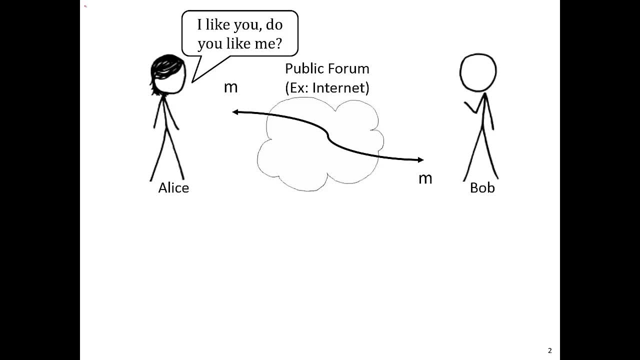 to send a note that says: I like you, Do you like me? And of course, Bob's reply is also potentially private. Now they're going to pass these messages across a public form, for example the internet, And the goal is to secure this communication. And of course we have to be secure against someone. And 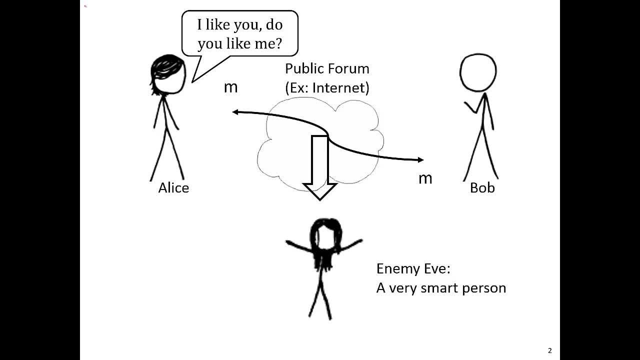 the way we model, that is, we come up with an adversary And we typically call this adversary, or enemy, Eve. This is actually short for eavesdropping, But in fact Eve can do much more than just eavesdrop. For example, Eve may try to 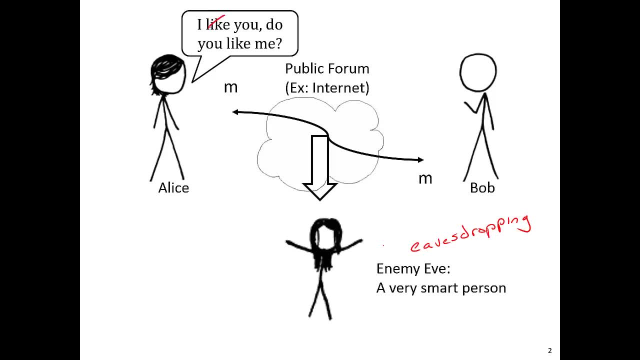 change the message. For example, instead of saying like maybe what Eve does is tries to flip the message to say hate. That would be catastrophic. So the goal of cryptography is to protect this communication, to make it secure. So in a sense, we want to come up with this notion of a 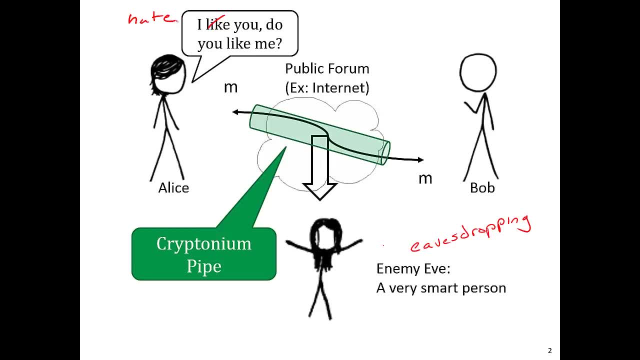 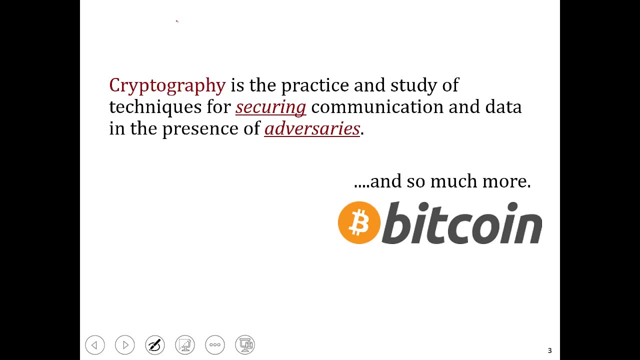 kryptonium pipe where Alice stuffs messages in the kryptonium pipe and Bob pulls messages out And they know that during transit Eve couldn't read, couldn't tamper, couldn't do anything to these messages. So a classic definition of cryptography is: cryptography is really the. 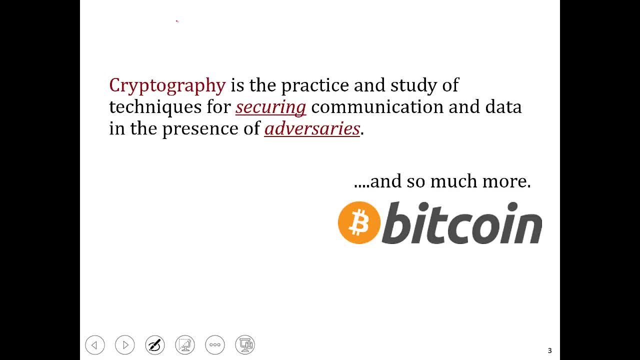 practice and study of techniques for securing communication and data in the presence of adversaries. Really, it's the science of coming up with this kryptonium pipe. But it's not just about securing communication and data in the way we normally think of it. It can actually be much. 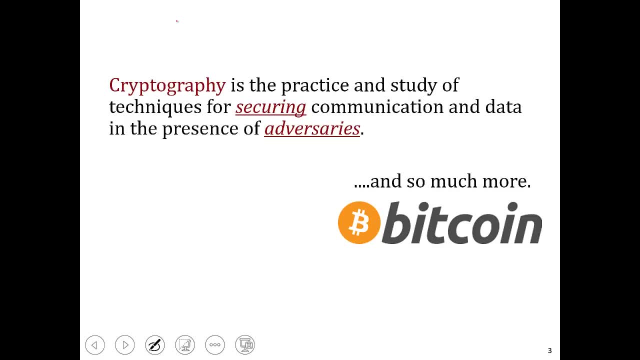 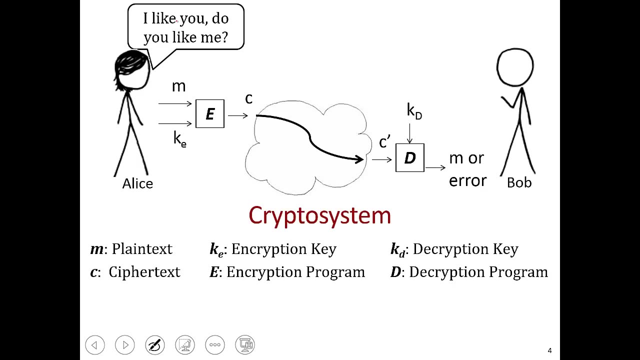 more. For example, cryptography is one of the backbone ingredients in a new internet currency called Bitcoin, So it's not just securing communication, it's actually creating a new opportunity for a new currency. Now, in order to describe how we come up with this sort of 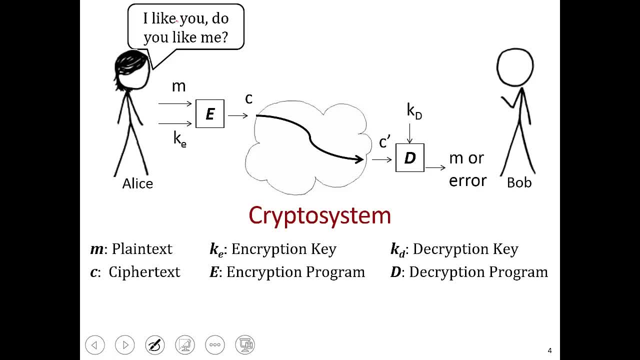 kryptonium pipe, we come up with something called a cryptosystem, And a cryptosystem consists of the different parts needed to communicate securely, And so at the core of the cryptosystem is an encryption program and a decryption program, And so the way a cryptosystem works is that it's a system of encryption and a decryption program. 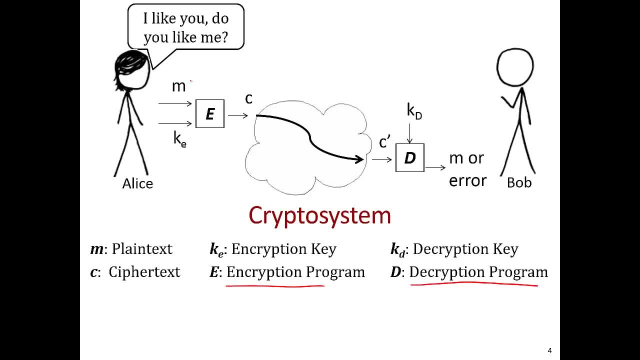 So the way a cryptosystem works is: Alice encrypts her plain text message, which I have here represented by M, by giving it to the encryption program, And she also gives a key, And I have here it labeled KE to denote it's an encryption key. So this plain text message, the original message, 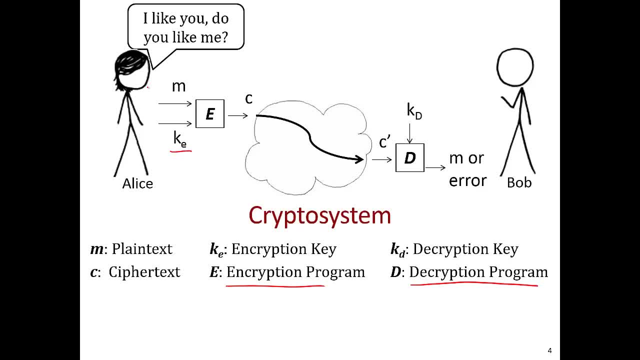 is fed into the encryption program and out comes a ciphertext And it's this ciphertext that goes across the public forum And in fact it's this ciphertext that Eve has access to. So Eve may try to eavesdrop or change the ciphertext or whatnot. So at the end of the public forum. 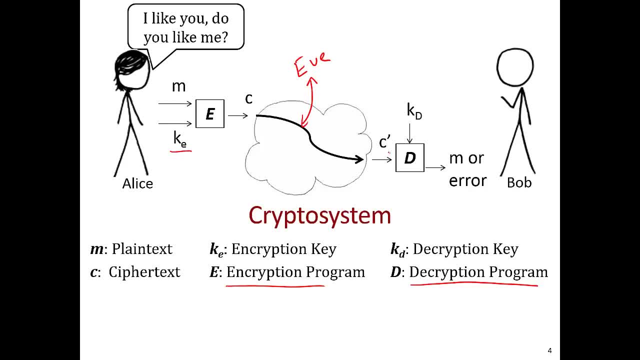 comes out another ciphertext And I've denoted this by C prime to indicate we hope it's the same thing as C but Eve may have tampered with it. So if Eve is tampered with it it's not quite the same thing. This ciphertext we receive, Bob decrypts with his decryption program and his decryption. 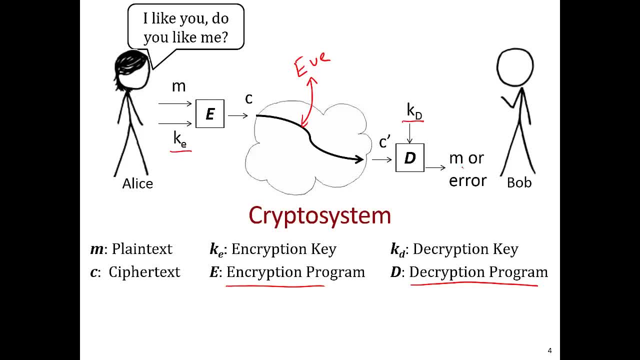 key KD, And what will come out is the encryption program, And what we'll see is that the encryption program is either an original plain text message M or an error, And in particular, this error is very important. Error is the way Bob knows that C was not equal to C prime, And so error is in a. 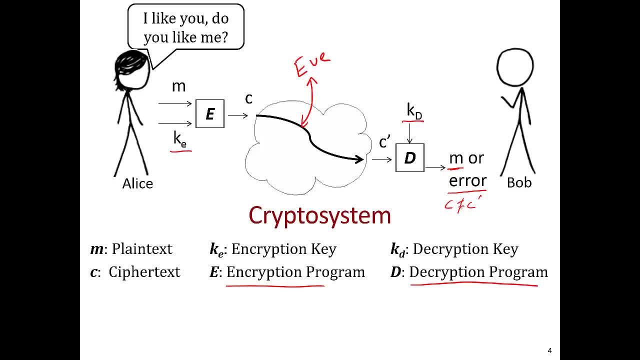 sense, what tells us if Eve has tampered with the message? Now there's some important things to note here. First, in modern cryptography, the security of the system purely relies upon keeping the encryption and potentially decryption key secret. So the security relies upon the secrecy of the keys and nothing more. In particular, we assume the 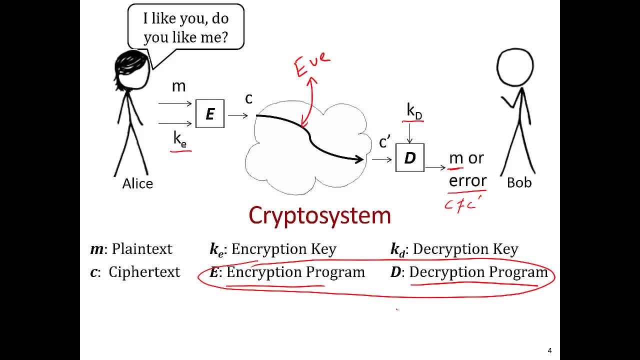 encryption and decryption programs are public. They're well known Why? Well, history has shown that trying to keep the programs themselves secret is really actually dangerous and doesn't work out very well. So we try to reduce security to the smallest thing, which is really just this key. The second thing: 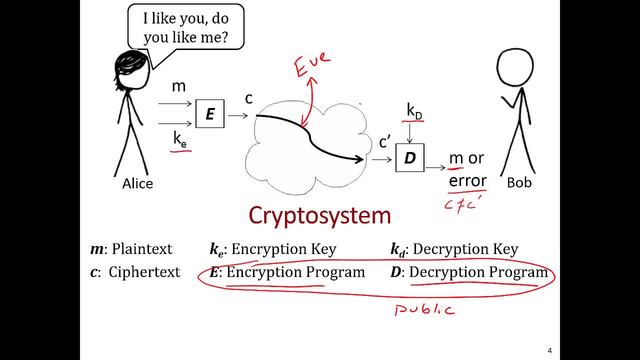 I want to note here is that I've seen a lot of people who have been using the encryption and decryption system. They've said there's two keys: There's an encryption key and a decryption key, And in fact in many classic cryptosystems these two keys are exactly the same thing. For example, this may be a shared 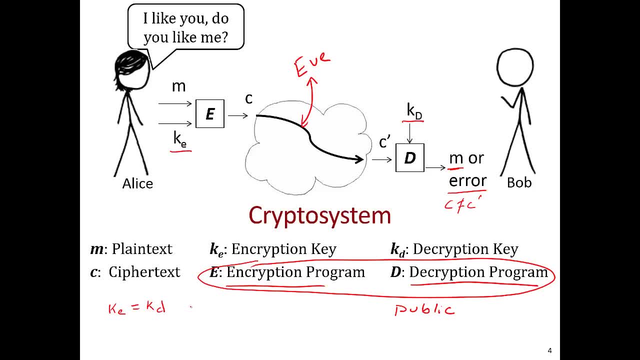 password. We call this private key communication, or another word that you may hear is symmetric encryption. Of course it's symmetric because both parties have the same key. It's also private, And one of the challenges with private key cryptosystems is the fact that both Alice and Bob know the same key. So either one of 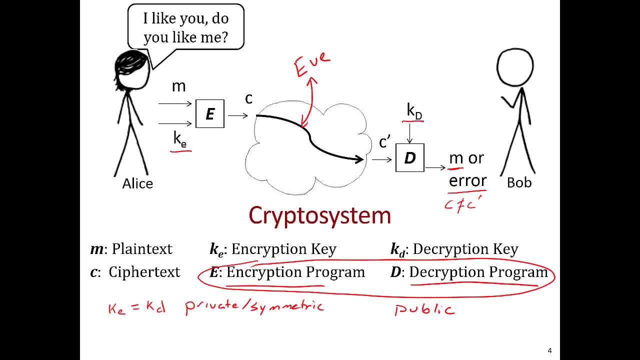 them by exposing the key can break the security of the cryptosystem In a sense. both Alice and Bob have to keep these keys well protected. One of the cool things that happened in the last few years is there's been cryptosystems. 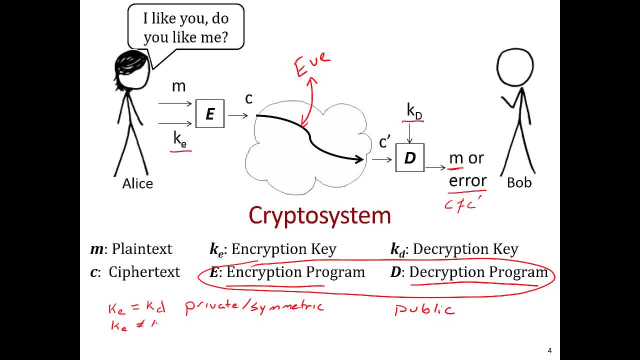 where KE, the encryption key, is not equal to the decryption key, And we call these public, or sometimes cryptosystems. Now, by asymmetric I mean that both parties don't share the same key. In fact, for example, if Alice wants to send an encrypted message to Bob, and one way of doing a public key cryptography scheme, KD is 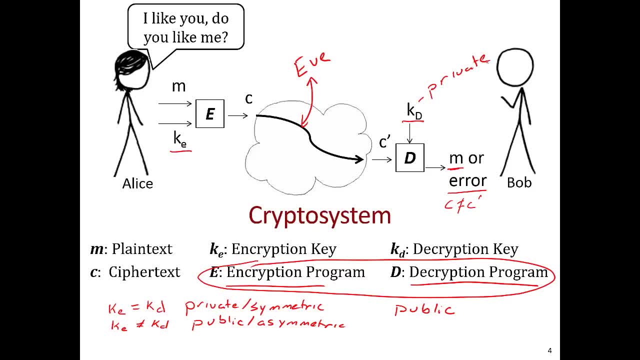 private, but Bob publishes a public encryption key to everyone. Now Alice would use this public encryption key to encrypt something to Bob and know that only Bob can decrypt it because of certain mathematical properties that make it so that only the holder of the private key can decrypt those messages. So this really took off around. 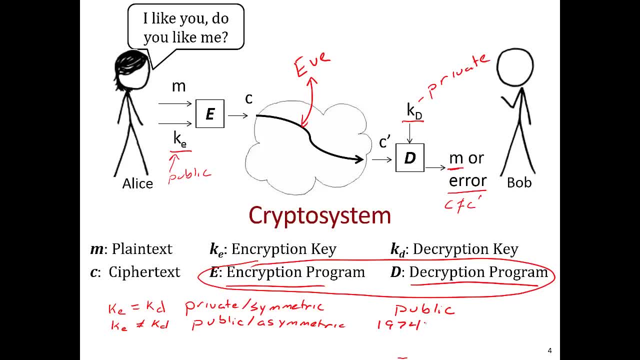 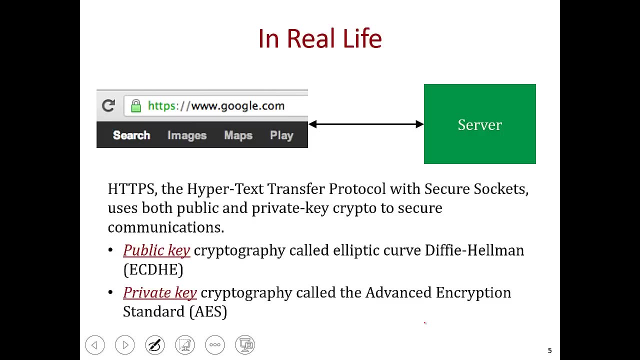 1974, when a variety of different people were studying this problem with. really, Ralph Merkle was probably the earliest, but there are other people like Diffie and Hellman and RSA, and even GE A, H, C, Q, which is a British spy agency. 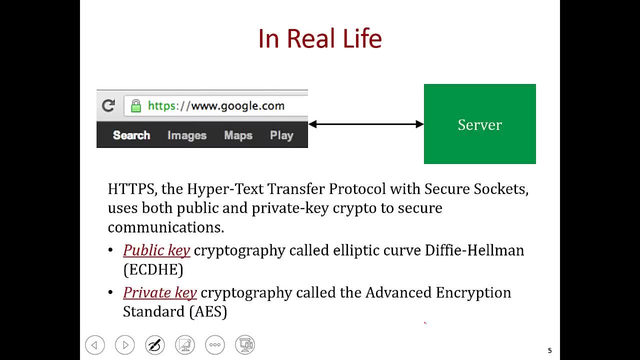 So in real life, of course we use both. We don't just use public, We don't use private. We actually use both public and private, And probably the most readily available example is HTTPs, which stands for Hypertext Transfer Protocol with Secure Sockets.